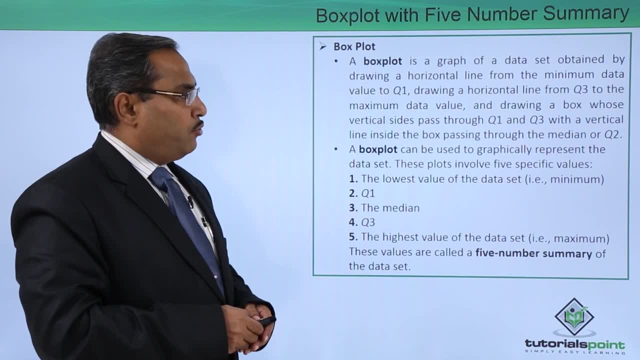 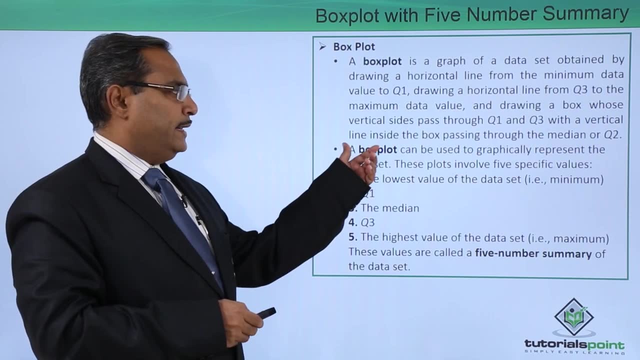 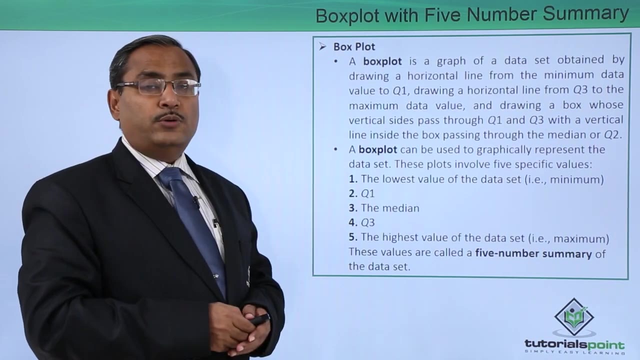 but quartile 1 and quartile 3, and drawing a box whose vertical sides pass through q1 and q3, with a vertical line inside the box appearing through the median, or q2.. So this is the q2 will be known as the second quartile, can also be called as a median. So a box plot can be used to 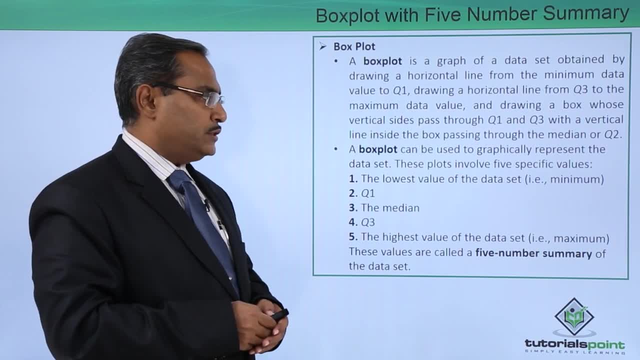 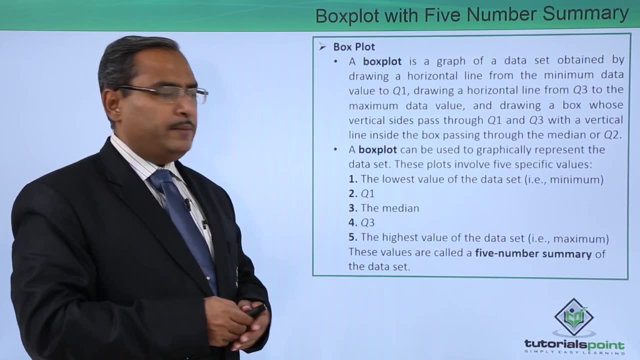 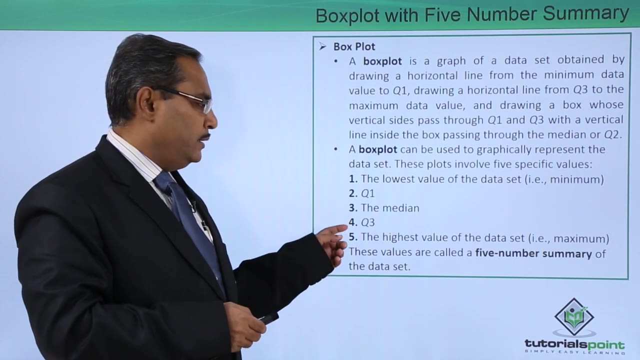 graphically represent the data set, and these plots involve five specific values. So the first one is the lowest value of the data set, that is the minimum. then we are having the first quartile, then the median also can be called as q2- second quartile. then we are having the third. 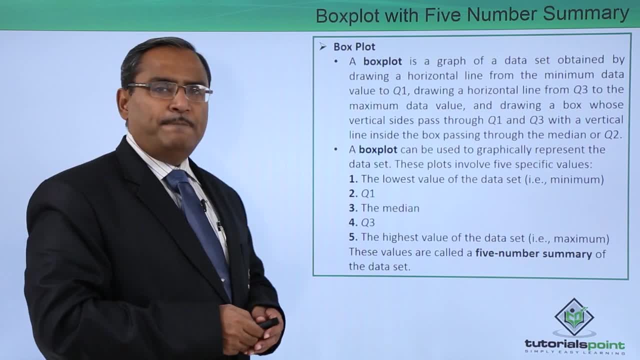 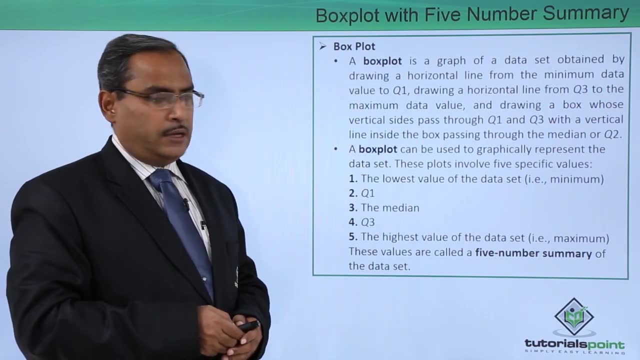 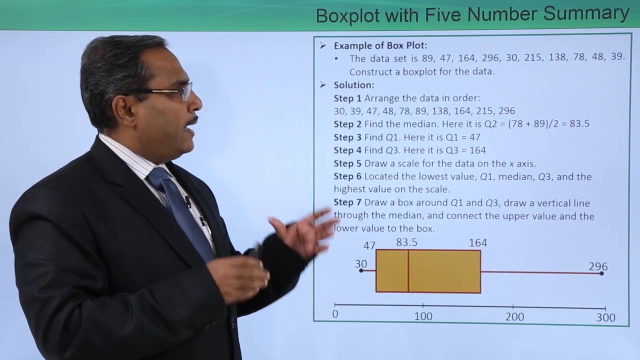 quartile q3 and the highest value of the data set, that is, the maximum. These values are called a five number summary of the data set. I think to make the conception clear we require one example to explain. Let us suppose we are having a box plot with five numbers. So we have a box plot. 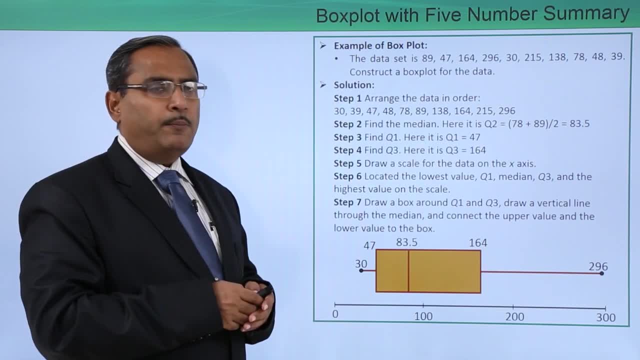 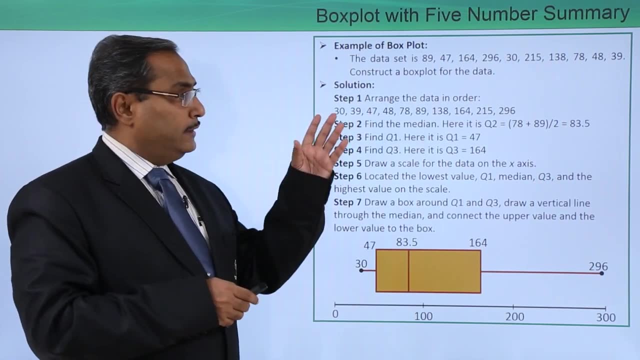 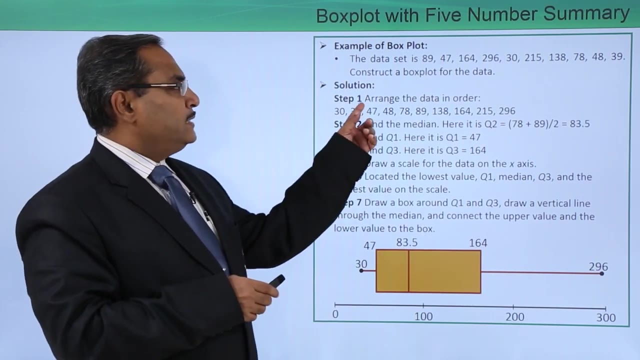 having one set of data on which we are supposed to draw a box plot. So the data set is 89, 47, 164. in this way, we are having this set of data and this data is not obviously shorted. Construct a box plot for the data. So arrange the data. that is a step number one. arrange the data in the order. 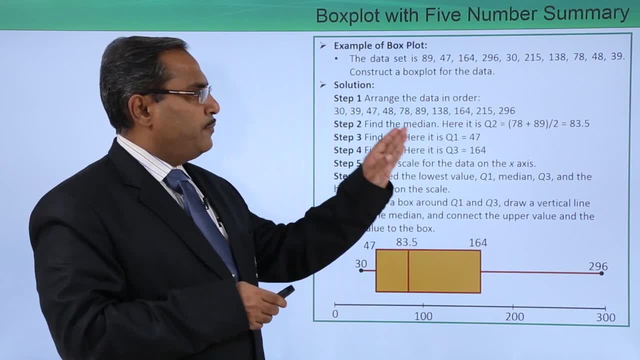 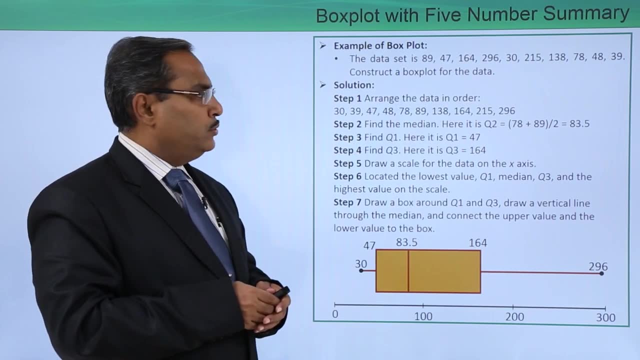 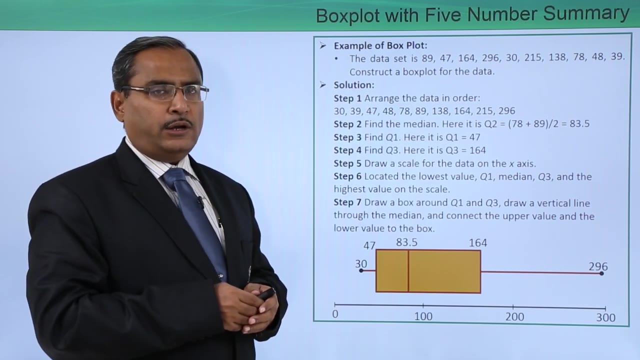 So from the, from the, from the lowest value to the maximum value. we have arranged all this data in the ascending order. Now step two, The median. We know that here we are having 1, 2, 3, 4, 5, 6, 7, 8, 9, 10 data. So 10 is even. So I cannot. 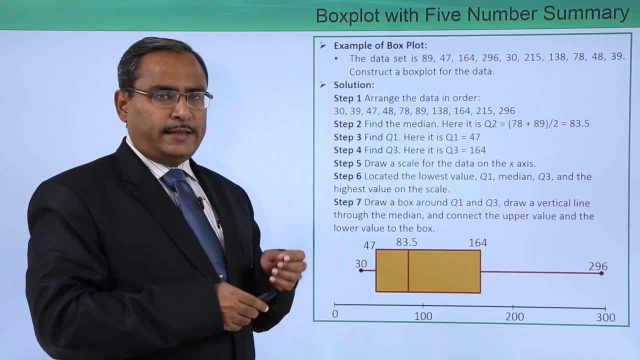 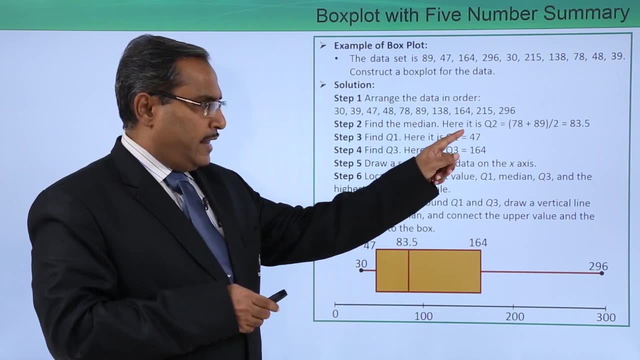 find the middle most value. So in that case I shall be taking the average of the fifth and sixth value. So 1, 2, 3, 4, 5.. So 78 and 89, that average will be. the respective median also will be. 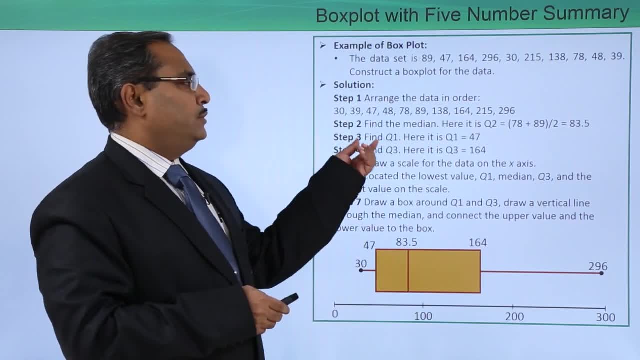 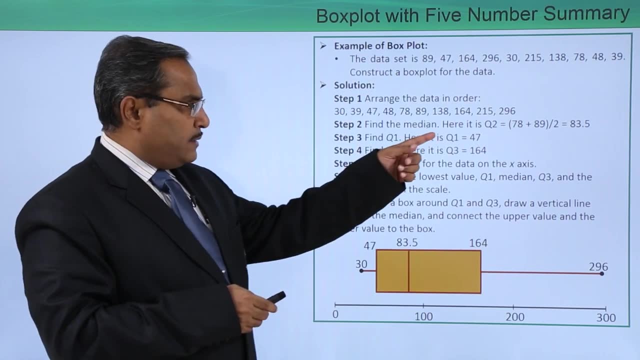 represented by q2 or the second quartile. So now we are going to find the q1.. So here we are going to find the q1.. So here it is. q1 is equal to 47.. What is the median here? That is 83.5.. So 83.5.